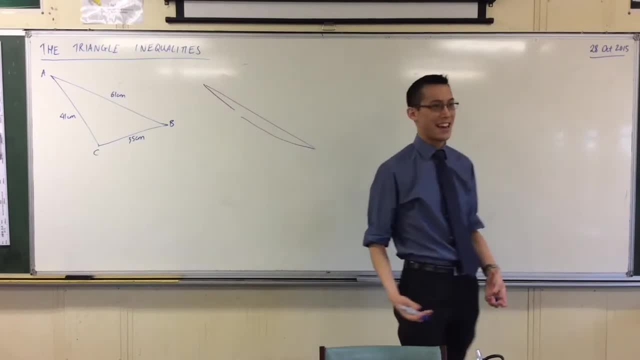 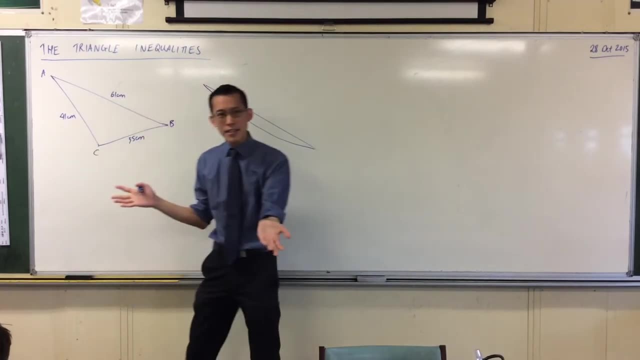 and AC would try and reach and they just wouldn't get there. So you can see, 61 has to be shorter than these two added together, And I can make the same argument actually for any of the sides of the triangle, This 41, it's got to be less than or equal to the sum of these two sides. 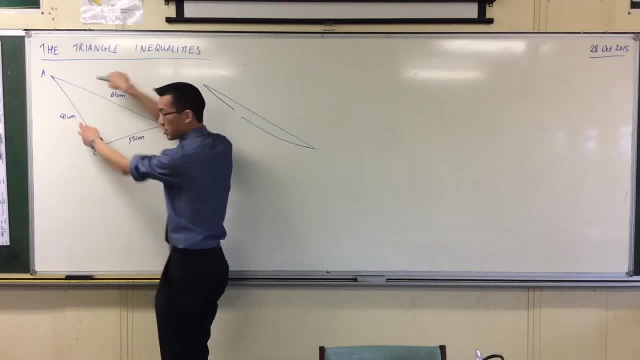 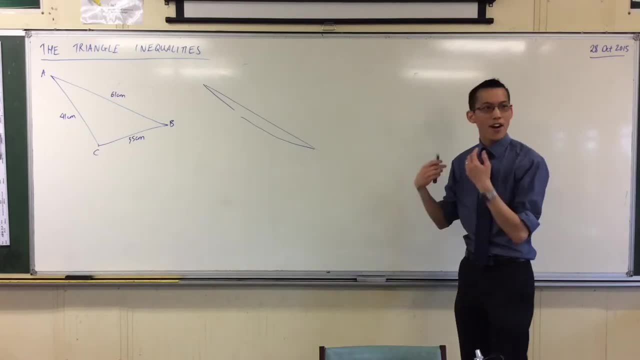 and 35 has to be less than or equal to the sum of these two sides, Otherwise your sides don't connect. you won't get a triangle. Does that make sense? Now, this is a very, very obvious fact when you're just looking at a triangle. 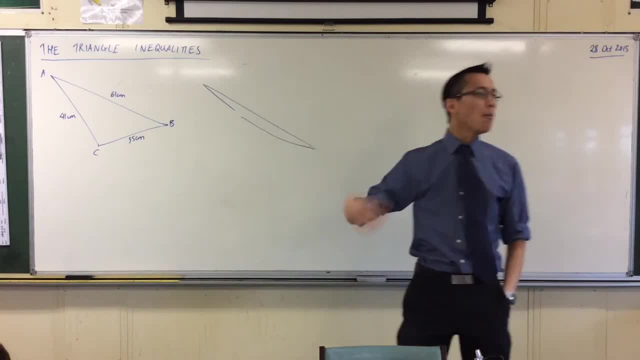 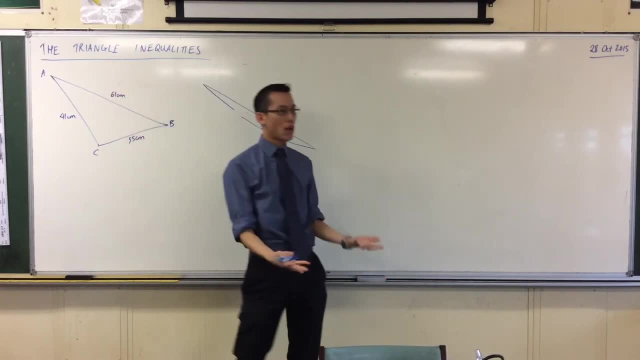 But the reason why I'm pointing it out here and the reason why I'm pointing it out now is because the whole point of thinking about complex numbers geometrically, if you remember, was that everything you know about geometry can then be applied to your complex numbers. 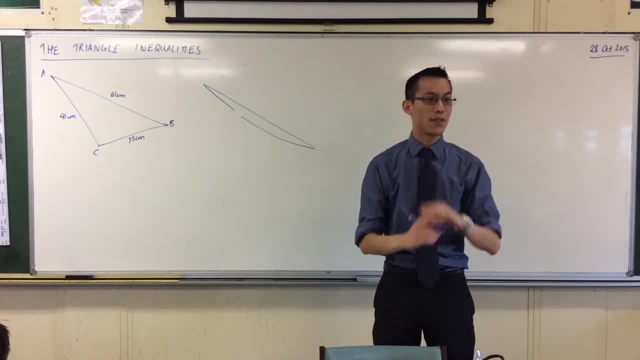 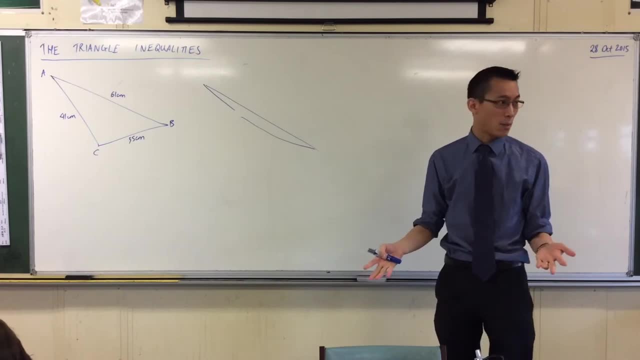 So I want you to have a think as I prime up my next diagram, and you can draw yourself a complex plane as well. Let's do it in the first quadrant for this first one. Triangles pop up everywhere when you think about complex numbers. 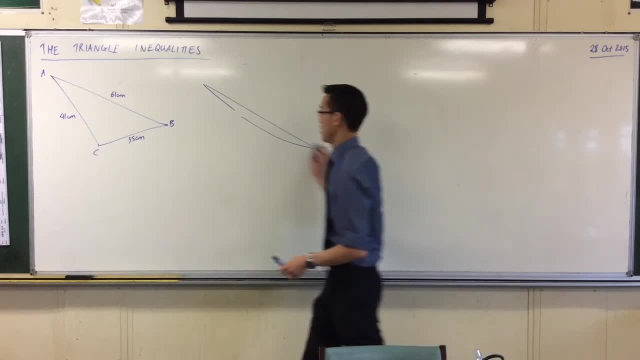 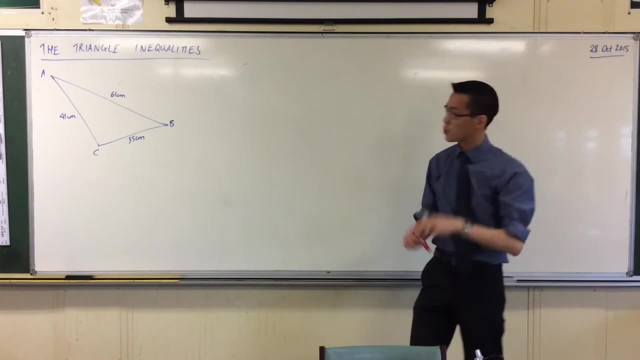 and how they relate to each other. In fact, there are already some very obvious relationships that we can have a look at which will take advantage of this. So, keeping that guy on the board, let's draw ourselves. we'll do it in the first quadrant. 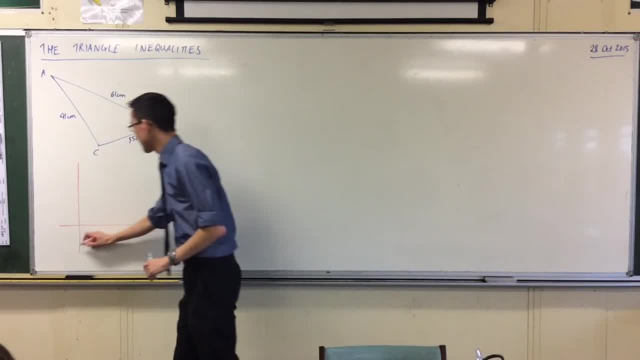 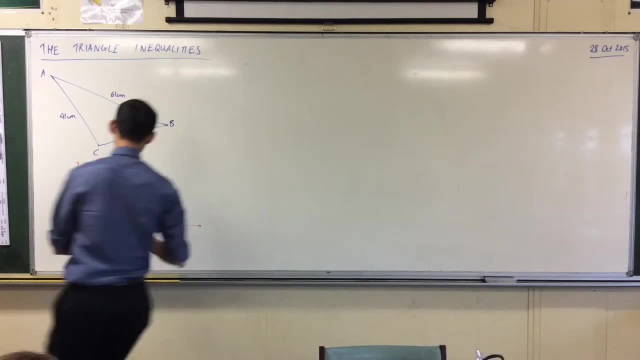 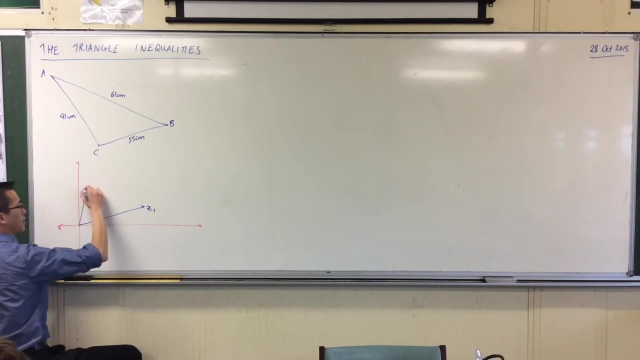 a complex plane like so And let's pop a Z1 and Z2 on here. We tend to do it something like this: Okay, Now the most obvious, first way to combine this, in fact, the way we've always been starting. 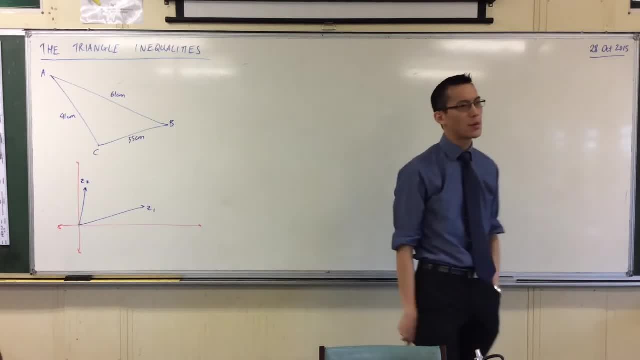 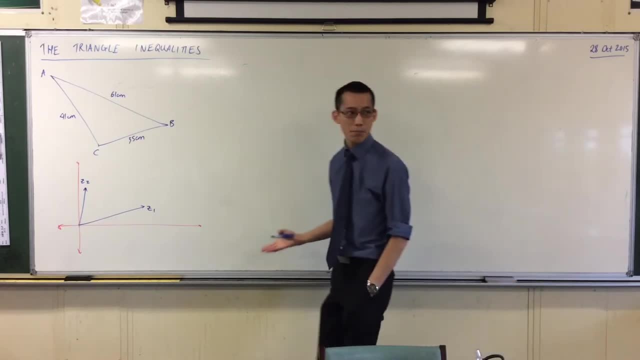 every time we look at a new idea is: let's think about what happens when we add these. Okay, let's think about what happens when we add them. So if I do Z1 plus Z2, where should Z1 plus Z2 be on this diagram? 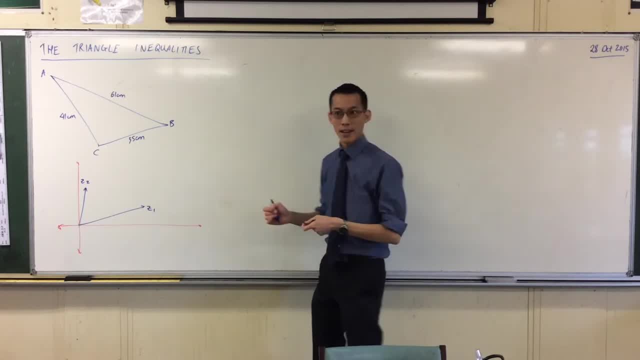 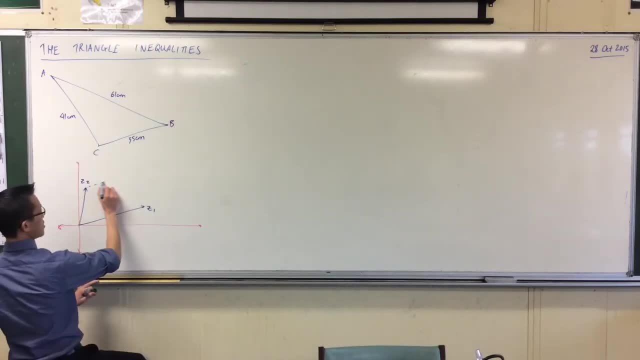 What shape will be formed when I plot Z1 plus Z2?? It'll be a parallelogram, right? because of the parallelogram law. So just in another colour I'm going to complete my parallelogram over here. So there's the parallelogram you can kind of imagine there in the background. 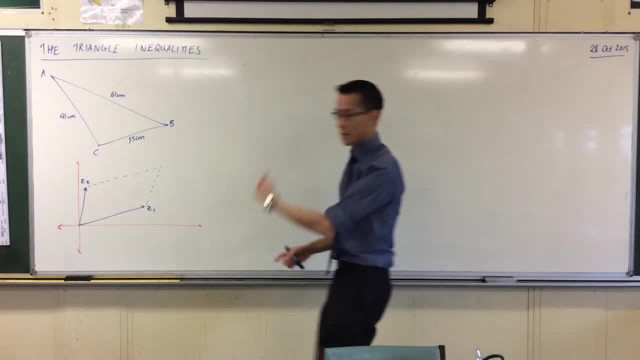 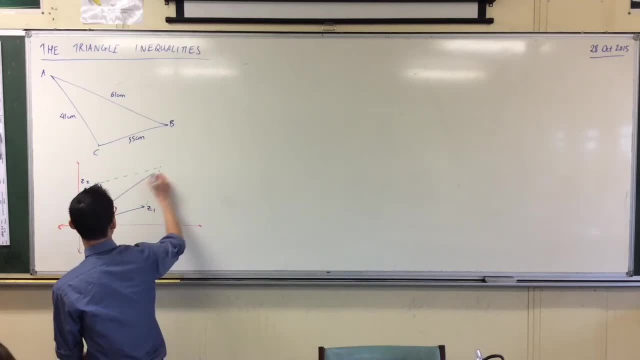 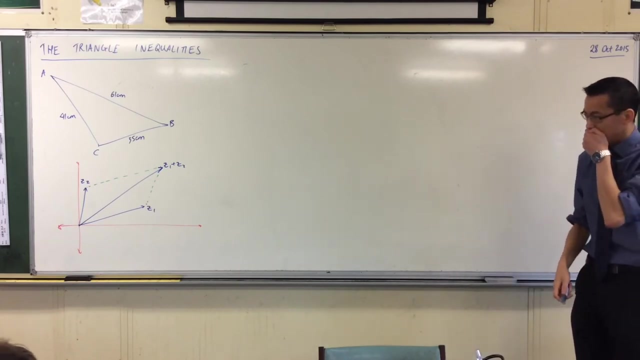 And Z1 plus Z2 is going to take you to the opposite corner. It's the diagonal. In this case, it's the long diagonal of this parallelogram. Okay so, Okay, now Excuse me, Because you've got this parallelogram right. 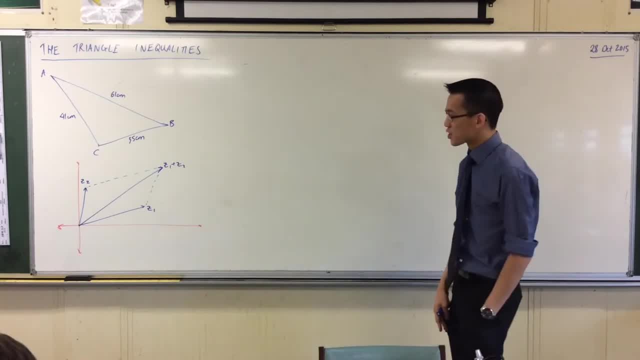 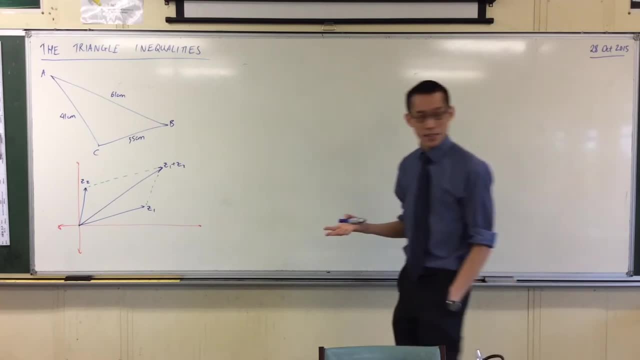 a parallelogram is made of a pair of triangles, So I can see in this diagram thinking about complex numbers not just as points but as vectors, right? For instance, let's have a look at this bottom half of the parallelogram here, right? 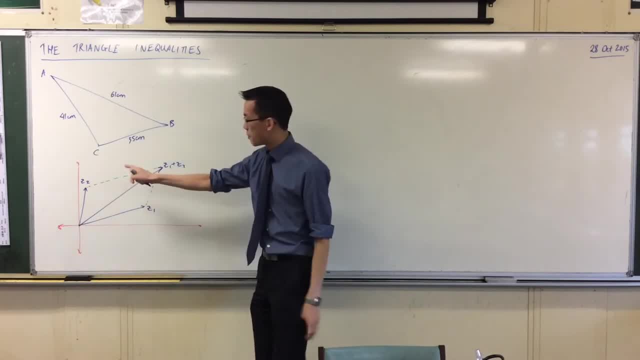 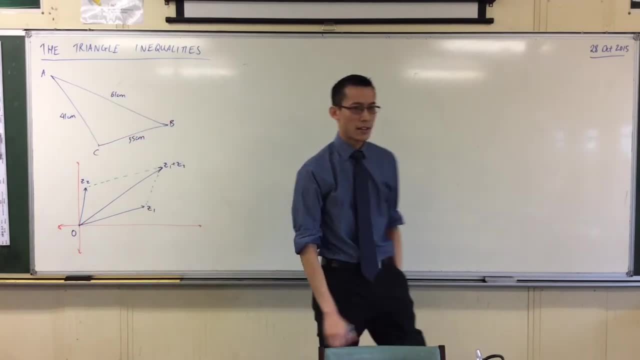 See how I've got Z2?? Think about that. That's the position vector of Z2 that I've got right there because it comes from the origin. Okay, there's the position vector, But if I consider one of the free vectors of Z2,, 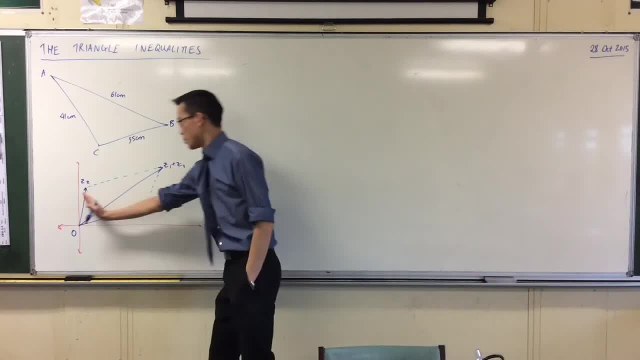 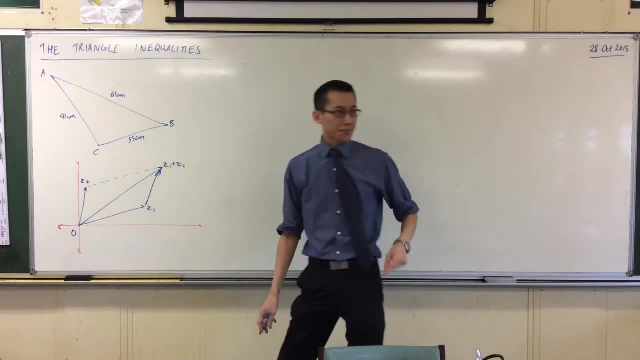 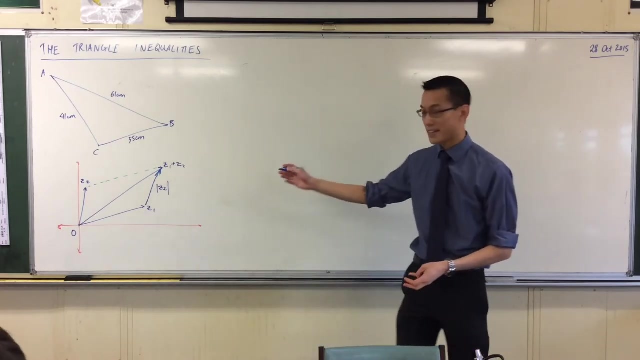 one of the free vectors that represents Z2, if I just move it to the opposite side, the parallel side of the parallelogram over here, okay, what I've got here is: this magnitude is the same, right, Because that free vector represents the same complex number. okay. 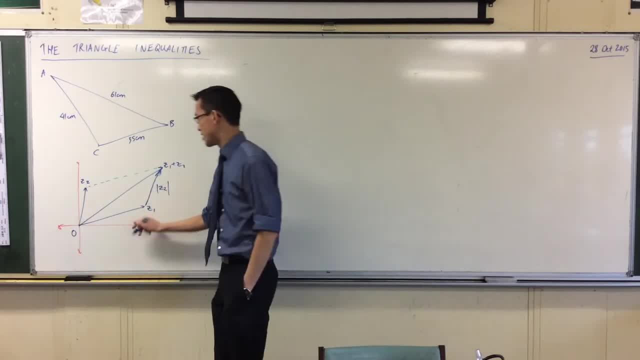 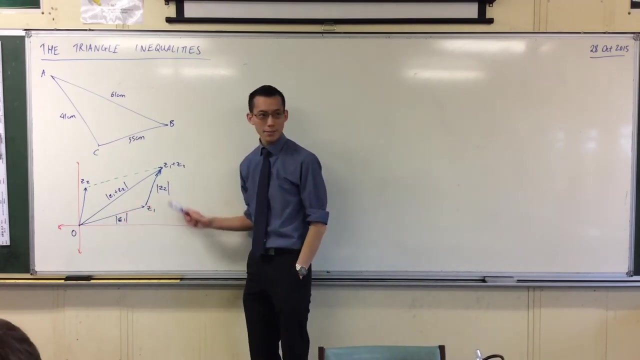 these lengths are going to be the same, So I've got a length over here. This is the position vector, so I've still got that magnitude there, And then that diagonal. its magnitude is the magnitude of the sum. Okay, So let's have a look at this triangle here, right, 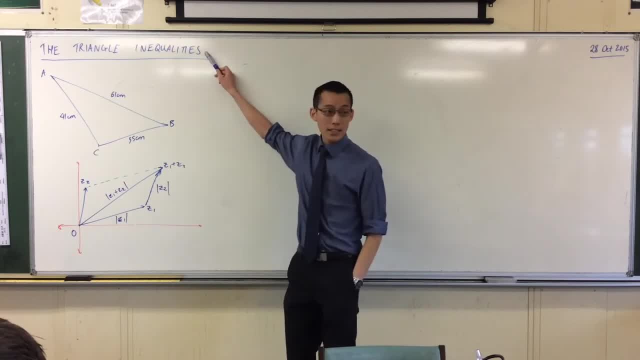 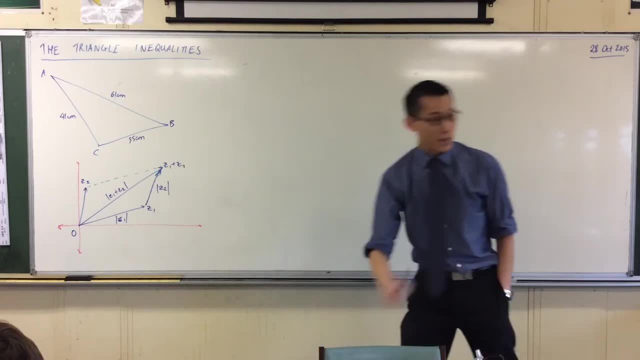 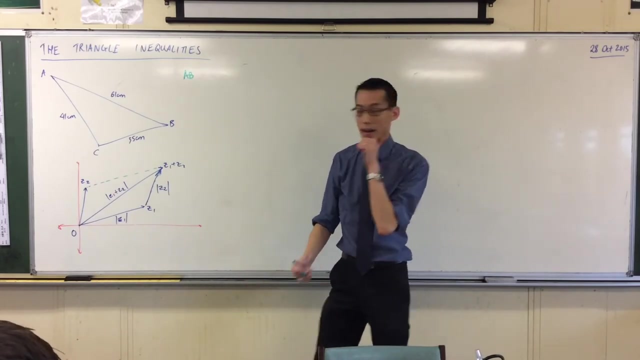 And what statements we can make in terms of inequalities based on this triangle here that are similar to what we said here. okay, So, for instance, let's come back to our original triangle, right, I can say that AB. right, that's one side of the triangle. 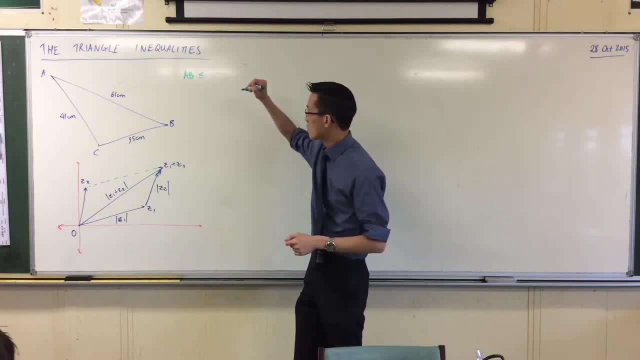 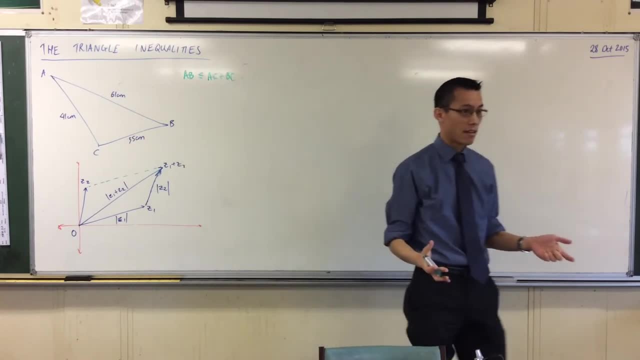 has to be less than or equal to the sum of the other two sides right AC plus BC. Do you agree with that Right? that's what we were saying before, Because if it were greater than, then the other two sides wouldn't be long enough to connect. 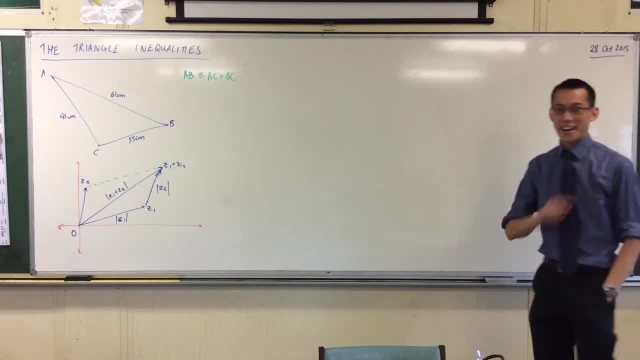 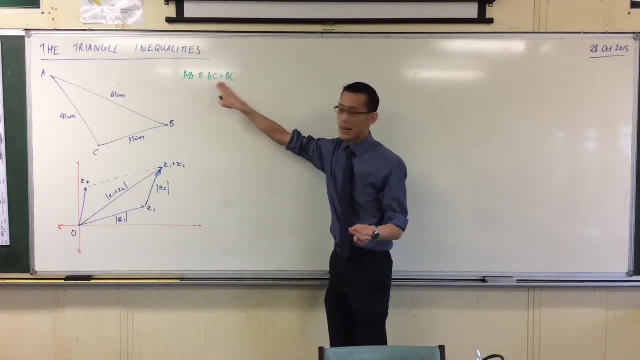 and complete the triangle. Yeah, Ah now. so that's a bit of a funny case really. What would happen if AB were exactly equal to the sum of AC and BC? That's kind of a bit weird, because in this context you wouldn't have a triangle anymore, would you? 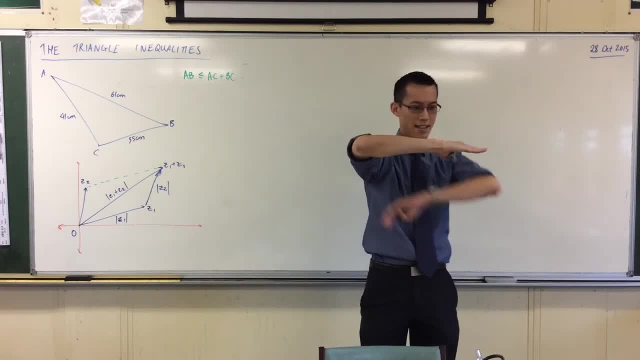 You'd kind of just have a straight line and there's the long side, and then you've got one of the short sides in here, and then you've got the short side there and they're just all sitting on top of each other. okay, But strictly speaking. 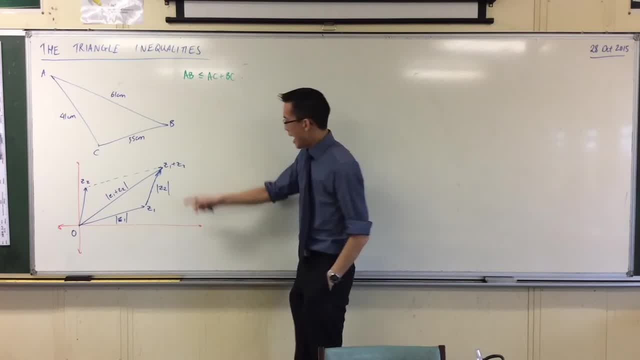 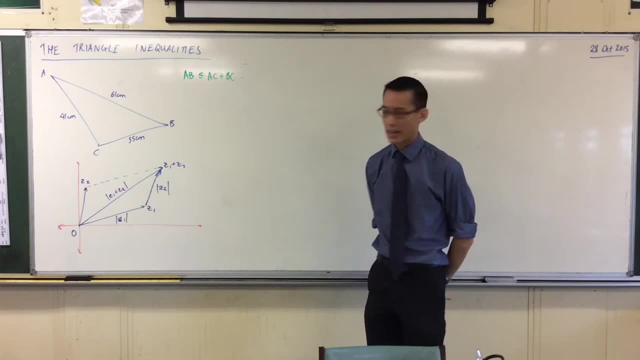 the lengths can still connect is what I mean. right, And in the context of a complex, a set of complex numbers, you can still have those and they can still. the intervals will still match up, okay, So that is a special case. 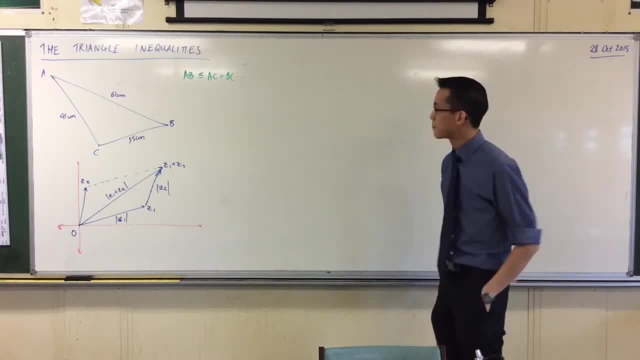 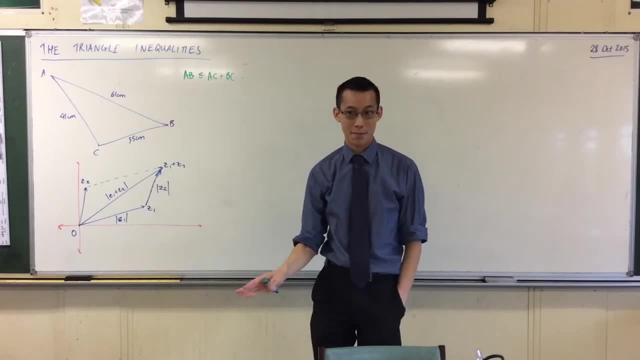 we'll talk about that a bit more in time, but I have to include it, okay, Remembering as well. I can say that statement not just about one side of the triangle, I can say it about any of them. alright, So there's one of them. 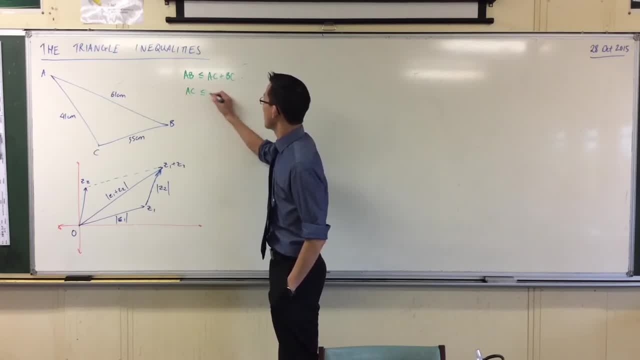 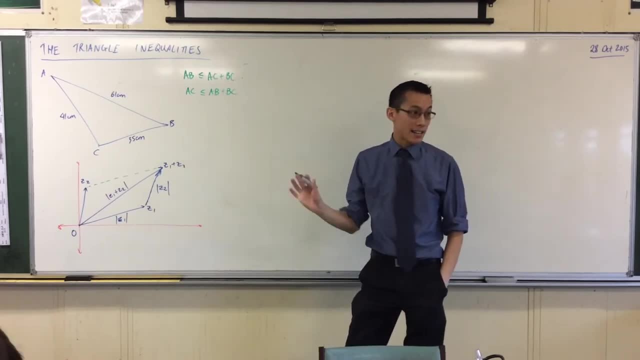 I can say it about AC. it's also got to be less than or equal to the sum of the other two sides, AB plus BC. and I can say it about the last side as well, which is BC. Okay, now, based on saying that, 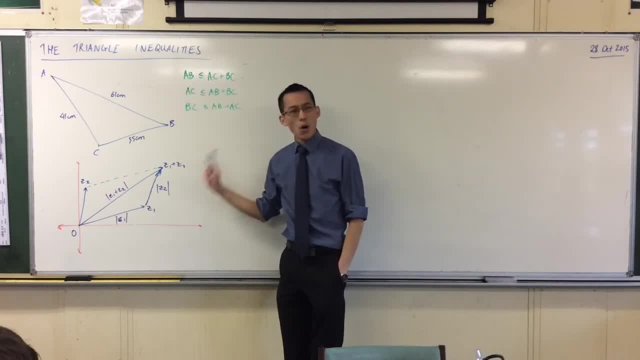 in our regular triangle up there. what equivalent statements can I make down here in this triangle? Let me just, let me just shade this in red so you can see the particular triangle I'm talking about. Okay, that's the triangle I'm interested in. 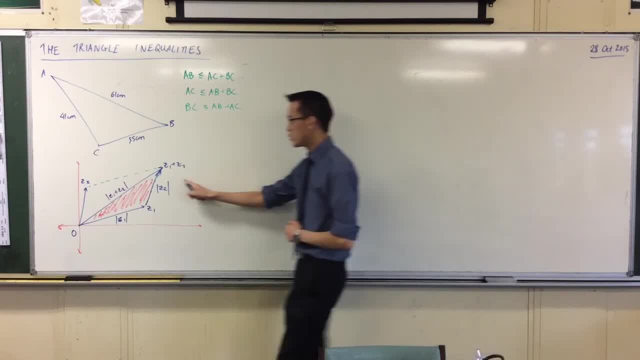 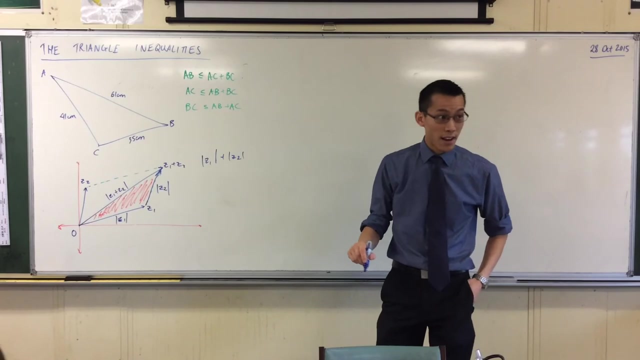 So what statements can I make based on the magnitudes of these lengths in this triangle? Yeah, give me one Equals. Okay, now I'm going to pause for a second, So I want to think about: yeah, yeah, yeah. 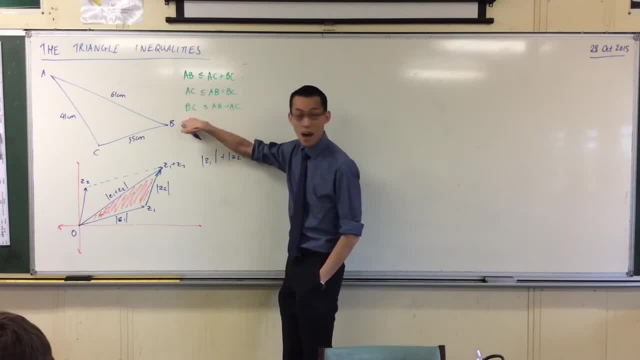 So I want to think about it in these terms: right, You consider one side, one side, and then you've got to say, based on the fact that I want the sides to connect, it's got to be less than or equal to. 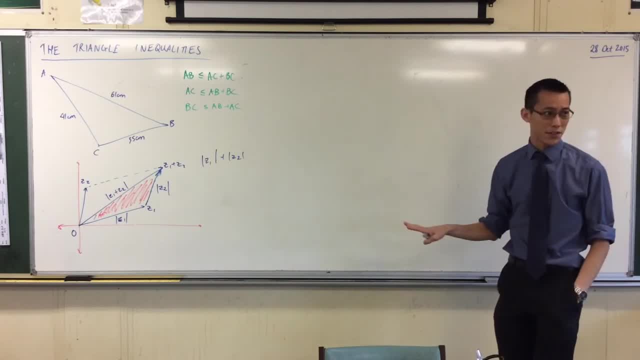 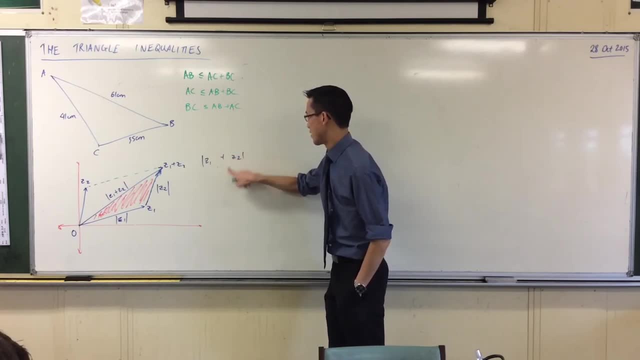 I can't say it the other way around, and in fact I will later on for a different triangle, but for here I'm trying to draw the parallel between here and here. I won't rub this off, I'll leave that there. 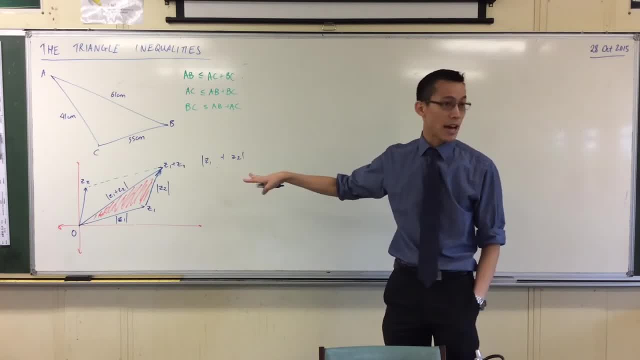 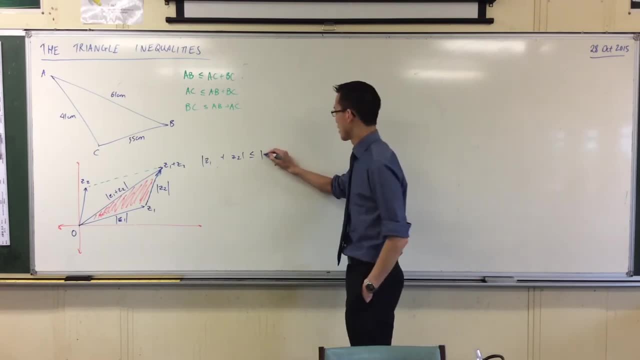 Okay, so there's a in this case, in my particular diagram, that's my longest side, okay, And it's less than or equal to the sum of the other two sides right, Z1, there's one of the sides. 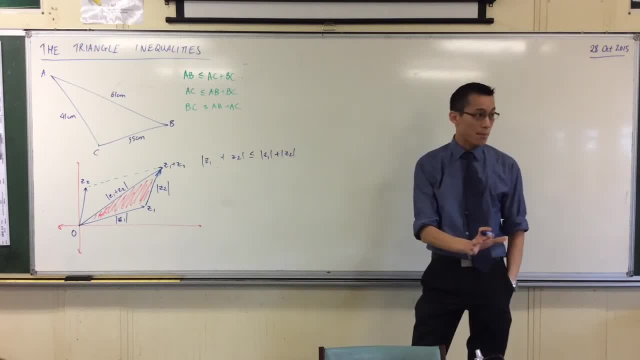 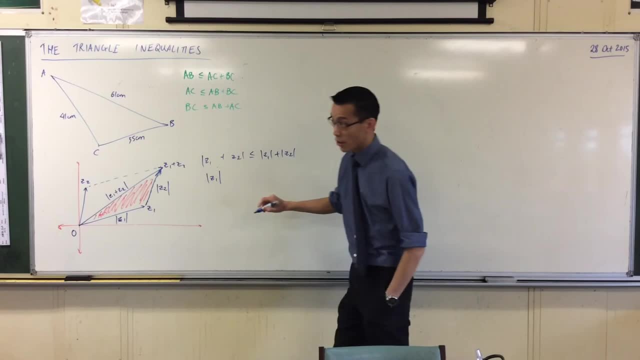 and Z2, there's the other one of the sides. Are you happy with that? Now I can just as equally say that for all of the other sides. right, I can say good morning. I can say that for Z1,. 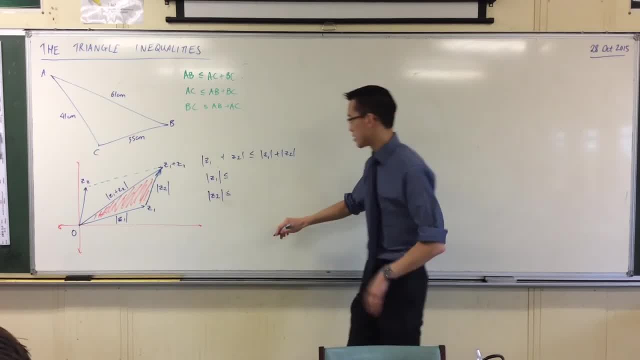 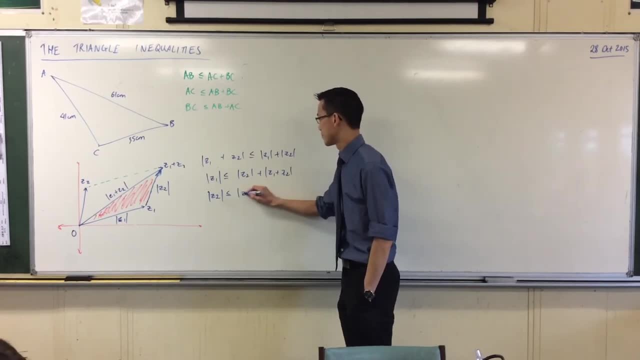 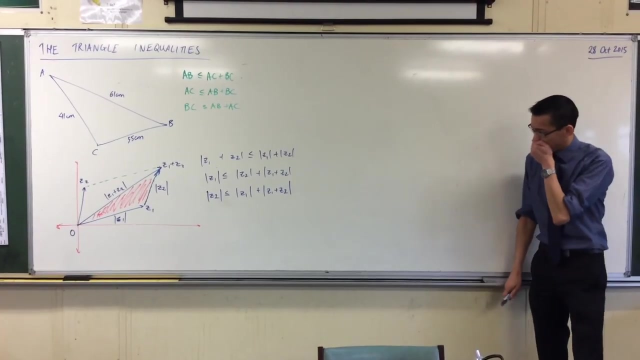 I can say it for Z2, right, And let's just complete this set of inequalities, Okay. Okay, there you go. Now, excuse me, these are all true. These are all true, Just like these are all true, Okay. 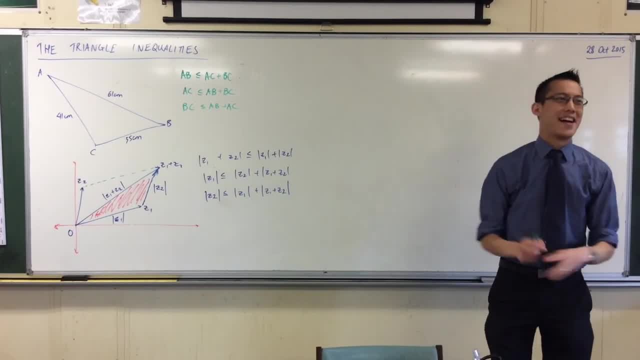 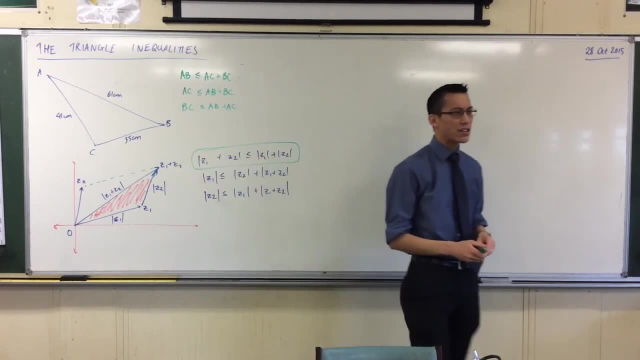 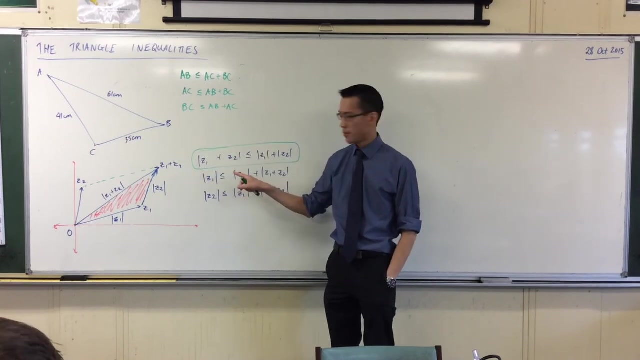 However, when we talk about inverted commas, the triangle, inequalities- okay, Can you see that this one here is kind of more interesting and elegant than the other two? Okay, It refers to the fact that the modulus of a sum, the magnitude of a sum of vectors. 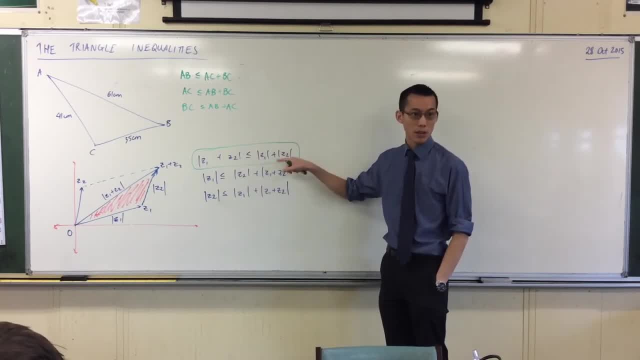 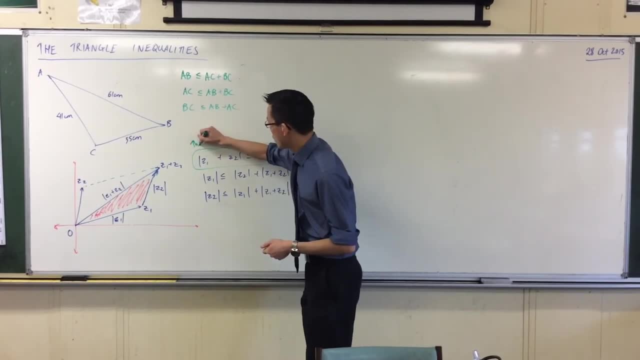 is less than or equal to the sum of the moduli of the vectors. Does that make sense? Right, Let me say that again. In fact, I'm going to write it, Okay: The modulus of a sum. the modulus of a sum. 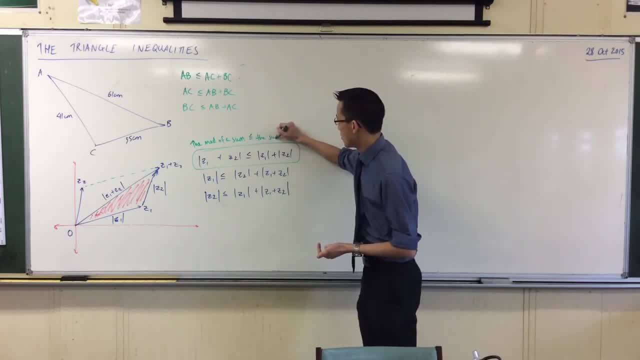 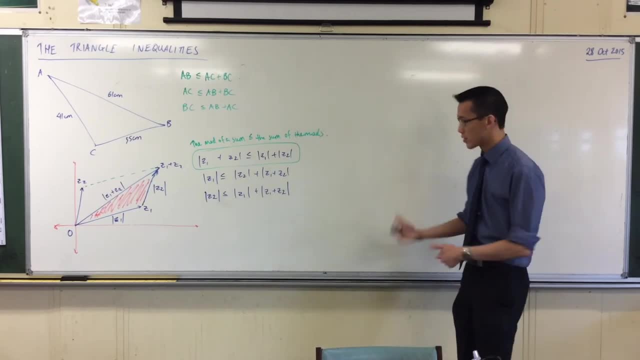 is less than or equal to the sum of the moduli. okay, The modulus of a sum is less than or equal to the sum of the moduli. okay. We're going to look at a concrete example of this in a second. 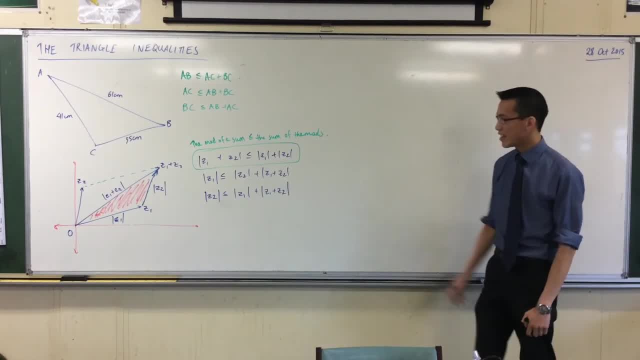 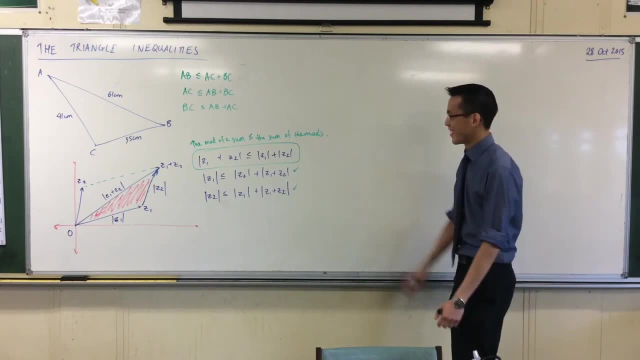 but this is all I want to establish for now. Okay, These are both true as well. Okay, They're just less interesting to say Okay. So this is my first result. Secondly, you remember in our parallelogram? 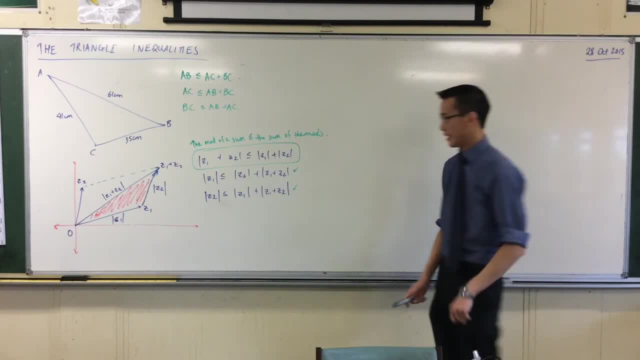 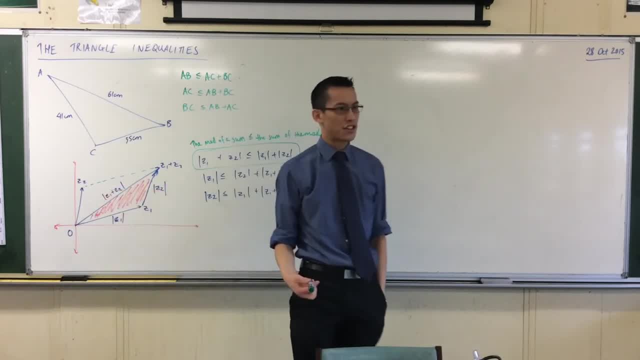 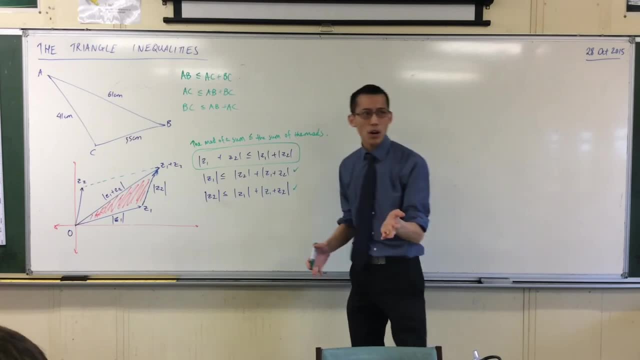 this triangle over here, this triangle over here. this triangle is congruent to the one I just said, So there's no more interesting stuff there, But there is another triangle based on the other diagonal. What's the other diagonal? What complex number.